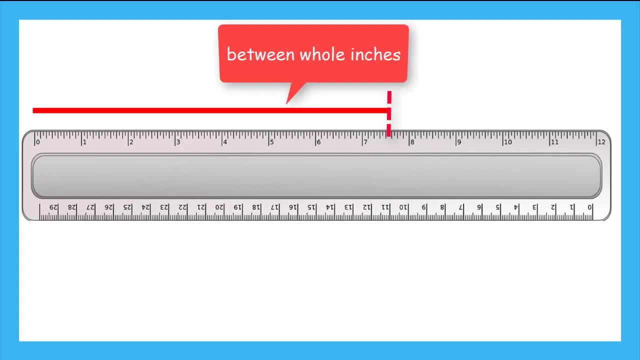 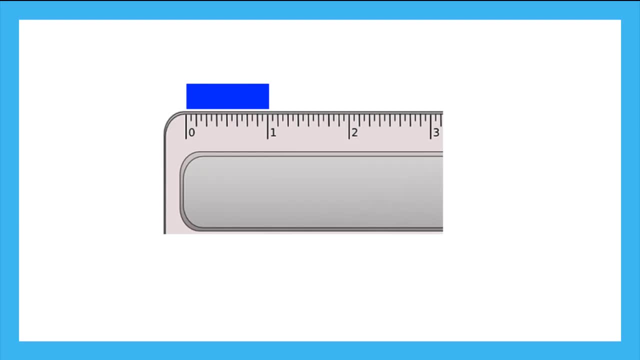 In this lesson we're going to learn how to measure things that are between whole inches. Let's start with inches. I've zoomed way in on our ruler here, so we only see the first three inches. Let's talk about what an inch is. This blue rectangle is one whole inch In the United. 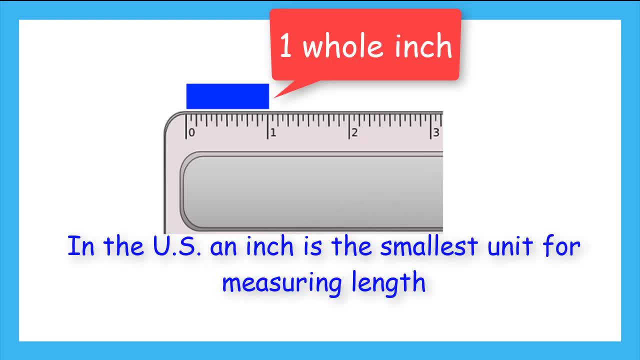 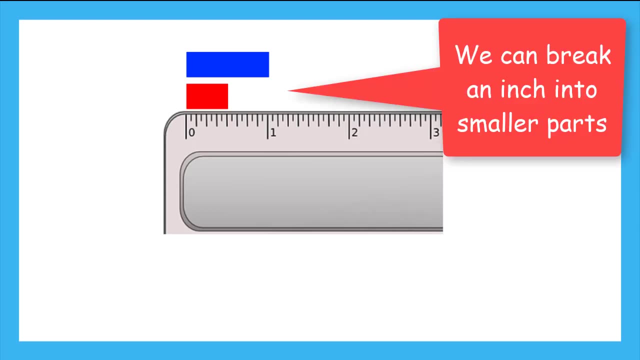 States, an inch is the smallest unit of measurement for length and height, But we know that there could be a rectangle that is smaller than one whole inch, Like this red rectangle. If we want to measure something that is smaller than an inch, we have to divide the 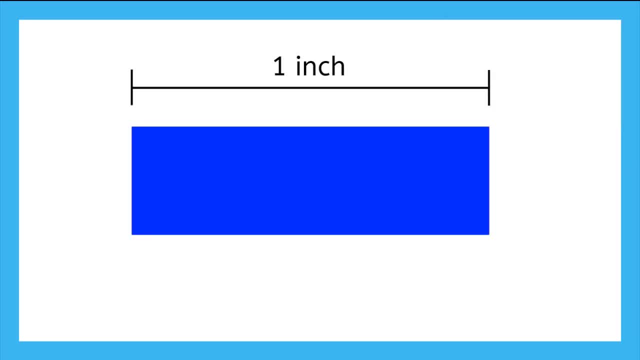 inch into parts. Let's use our blue rectangle to help us see. Remember, we measured our blue rectangle to be exactly one whole inch. Now, if we draw a line right down the middle of our rectangle, what do we get? Well, now we have two rectangles that are each half an inch. 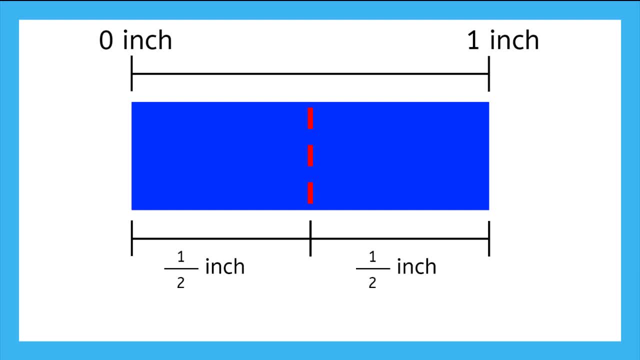 We can divide an inch into two parts that each equal half an inch. Now what if we draw a line right down the middle of both of the half rectangles? Now we have four rectangles. Now, using what we know about fractions, if we take one thing and divide it into four parts, 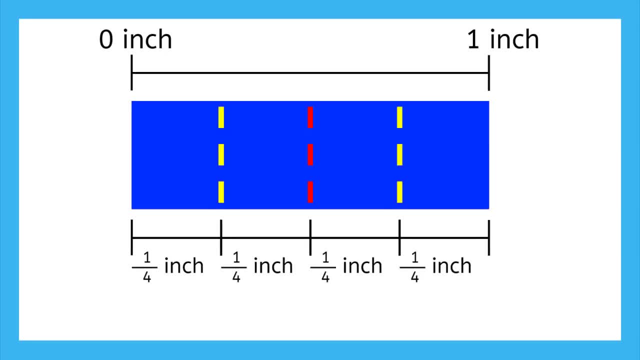 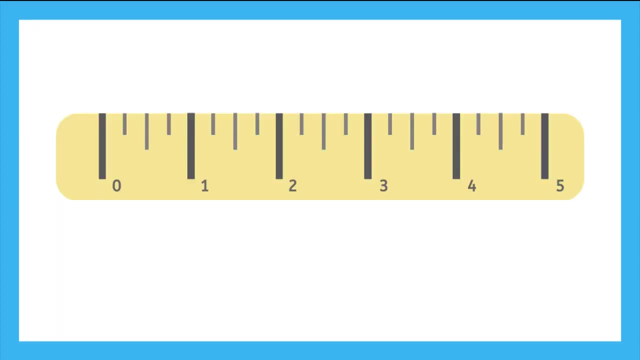 each part is one fourth. This shows us that we can divide one whole inch into four parts, And each part will be a fourth or a quarter of an inch. Now let's take a look at the ruler again. Do you notice anything about the marks on the ruler? Yeah, these big lines here. 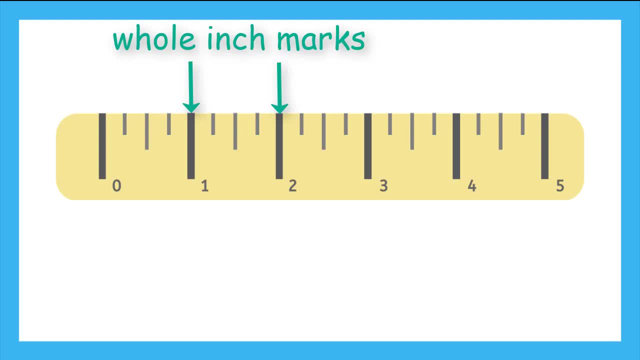 represent a whole inch. And then we see these three smaller lines in between. What do you think that this longer line in the middle represents? Well, if we compare the distance from the taller middle line to the whole inch lines, it appears to be right in the middle. So this is the half inch mark And these shorter lines. 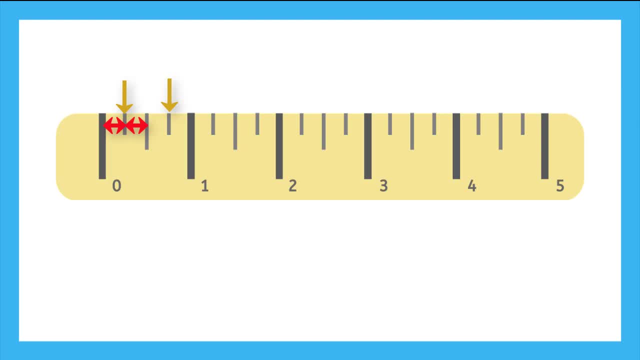 are cutting halfway between the half inch mark, so they must be the quarter inch marks. Let's zoom in now between the one and two inch marks and do a quick fraction review. Remember, each of these distances is one fourth, So if we're going to count them, we would have 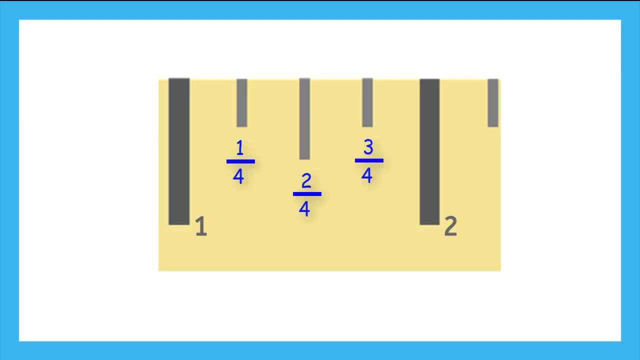 one fourth, two fourths, three fourths, before we would come to the next whole. And we can simplify two fourths to what? Yeah, that's right, a half. Now that we know how to divide an inch into parts, let's measure the length of this green line. 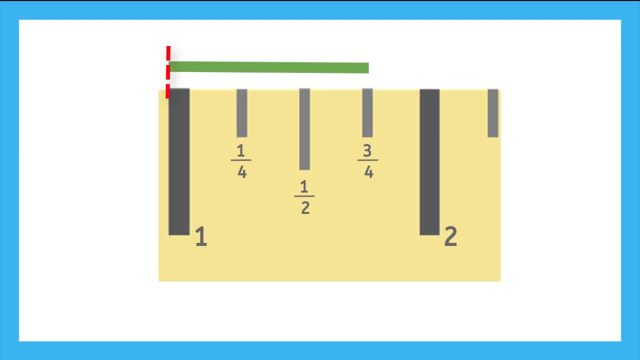 So if it starts here at the edge of the inch mark and it goes a quarter, a half, three quarters across the inch, this green line is three quarters of an inch. Let's do a few examples now, without looking at the numbers. 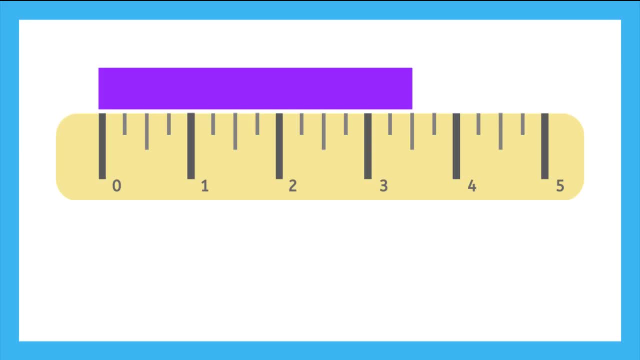 our extra markings. What is the length of this rectangle? It starts at zero and it goes past the three whole inch mark. but by how much? Well, let's count: We have three and a quarter, three and two quarters, and three and two quarters is. 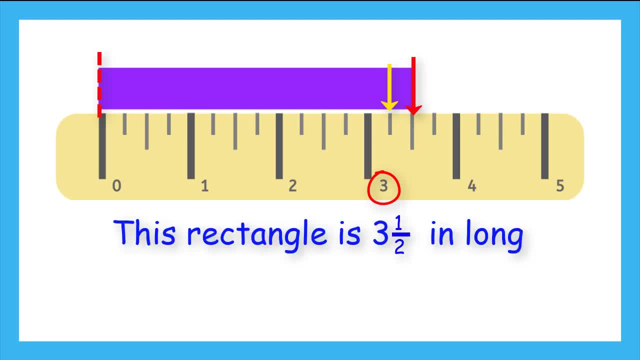 the same as three and a half. So this rectangle is three and a half inches long. How about this one? It's longer than the four whole inch mark and goes to the first marker, which we know is a quarter. So this rectangle is four and a. 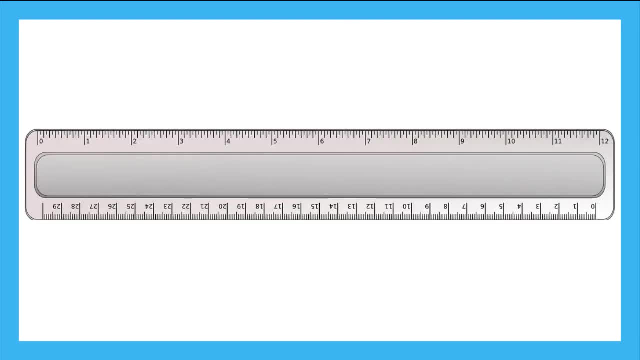 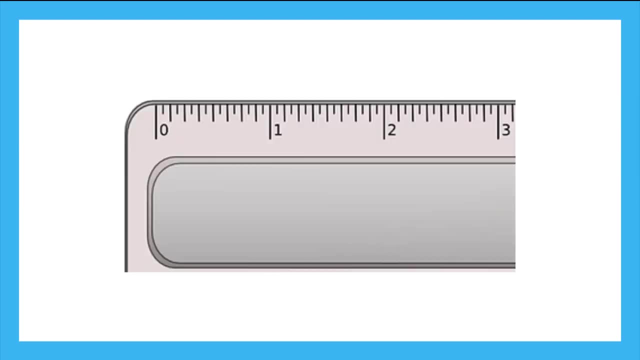 quarter inches long. Now let's take a quick look at our original ruler and find the half inch and quarter inch marks. We can zoom in to make it easier to see. Now notice, between the one inch and the two inch marks is・ marks. we have all these little lines. Let's count how many longer lines there are One. 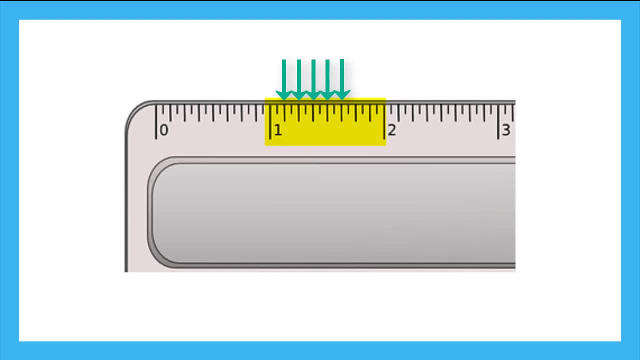 two, three, four, five, six, seven and one would make eight. So the halfway point would be at line four. If this is the halfway point between one inch and two inches, we know that this is the half-inch mark, And if we cut our half inch and half, we find the quarter.